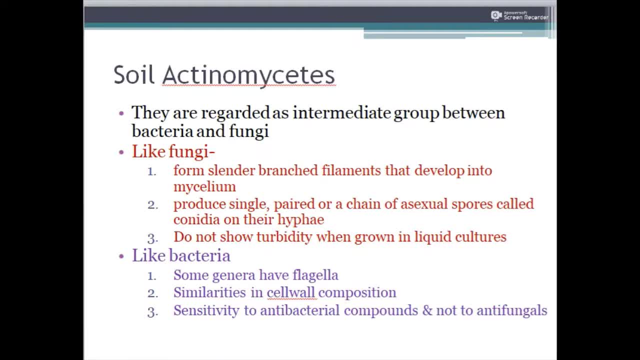 appearance. So normally, if you go to think about actinomycet itself, it has been found to be a very slow growing group and it has been found to have some of the properties of fledge of fungi as well as, at the same time, some properties of the bacteria. So if you have bacteria and if you have 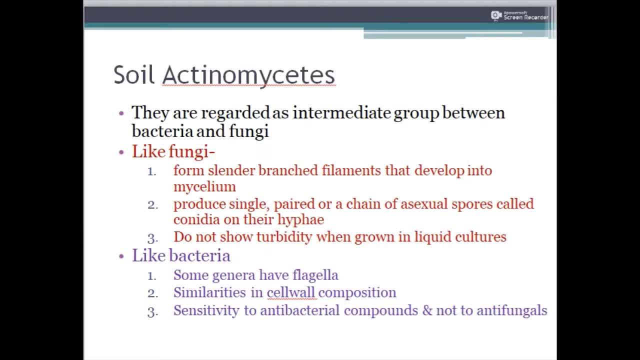 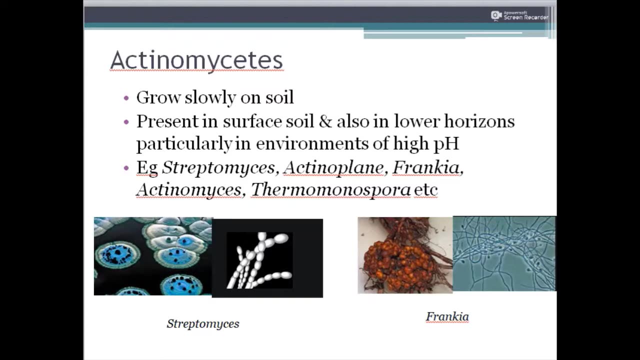 some of these bacteria. you are going to see that they have some very strong adverse effects on the health of the fungi. You keep actinomycets in between as an intermediate group, and let's talk about the actinomycets which have been found in the soil. 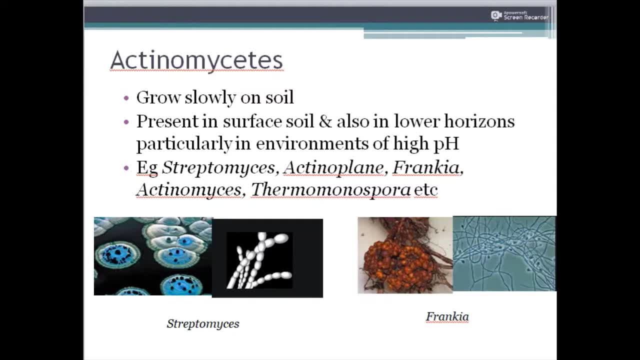 As we mentioned earlier, actinomycets. they have been found to grow at a very slow rate, and they can be present either on the surface of the soil, and sometimes they might also occur in lower horizons, particularly in the environments of about high peat. 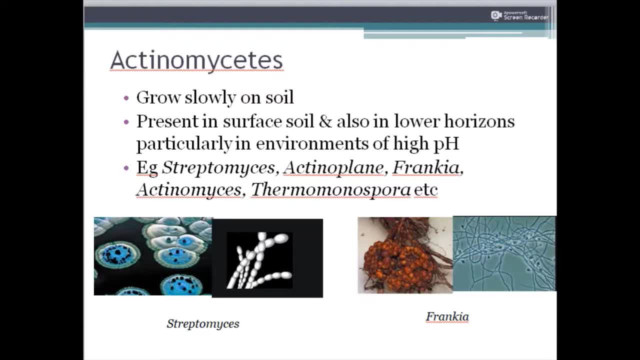 there are lots of a wide range of actinomyces in the soil, and some of the most important ones include streptomyces, actinoplane franquia, actinomyces thermomonospora, etc. these are some of the widely available actinomyces in the soil, and hope so you remember streptomyces, which is 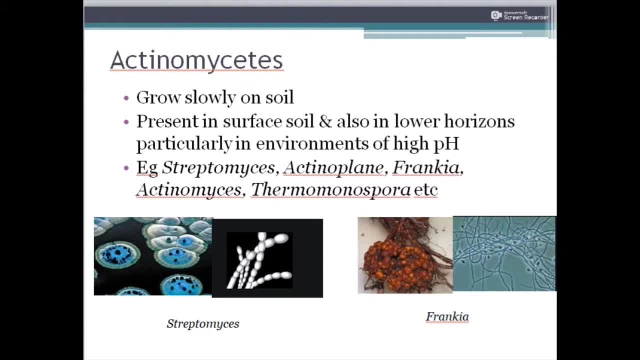 the responsible for the production of the antibiotic streptomycin. now, this is a culture plate growth pattern of streptomyces and this is how it looks when it has been viewed under the microscope, because it is filamentous and it will be from a filamentous bacteria. it's a 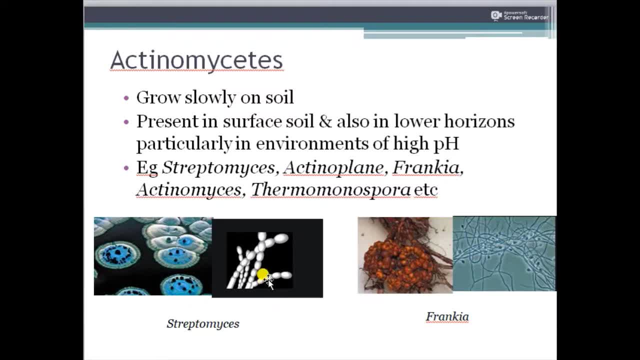 filamentous bacteria which will grow, but if you look at this, it will look like it is a fungus also, but it is a bacteria. another example of it is of actinomyces. it is franquia. when you look at this, you can- i think you remember this- has been found in the root nodules of some higher plants. franquia is a. 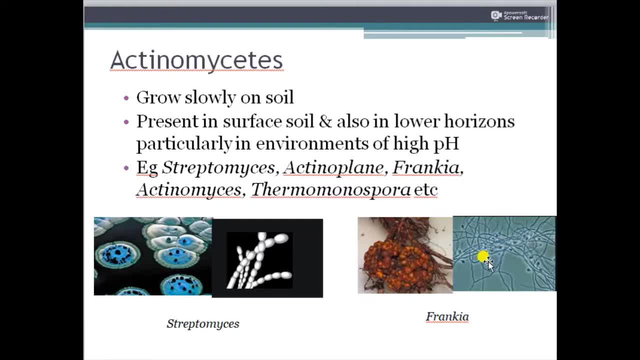 nitrogen fixing actinomyces, and under the microscope it looks like this: okay, so a various range of- and if you go to look, it's not easy to find out and by heart, all the actinomyces which have been found in soil, because actinomyces are a group of bacteria which have been found to be 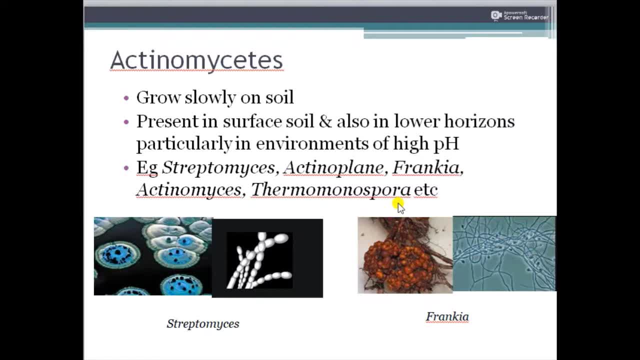 very vast and even now many of the actinomyces still remain unexplored to our knowledge. so but do remember the most important ones, such as streptomyces, franquia actinomyces, etc. and streptomyces of much importance because we have medicinal implications of this particular actinomyces. 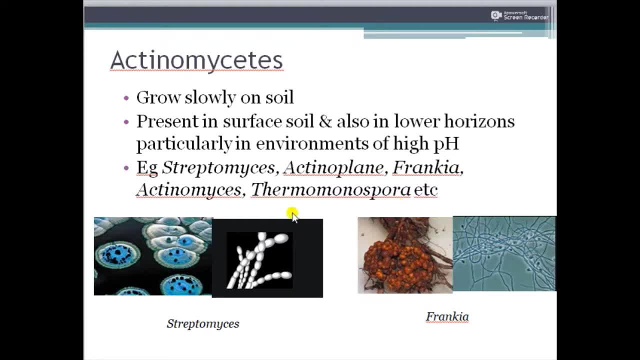 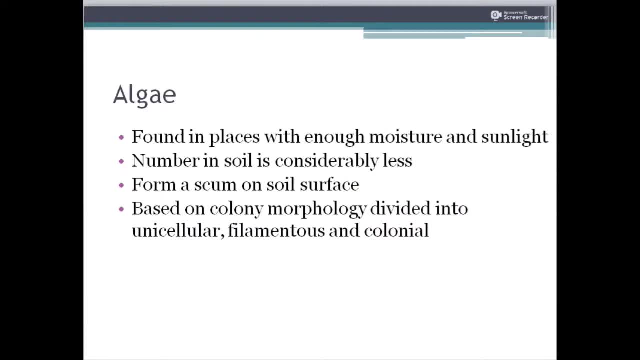 these actinomyces are usually slow growing ones. now let's talk about another microflora of the soil, referred to as the algae. these algae: they are found in places with enough moisture and sunlight, and their number in the soil is being found to be considerably less. 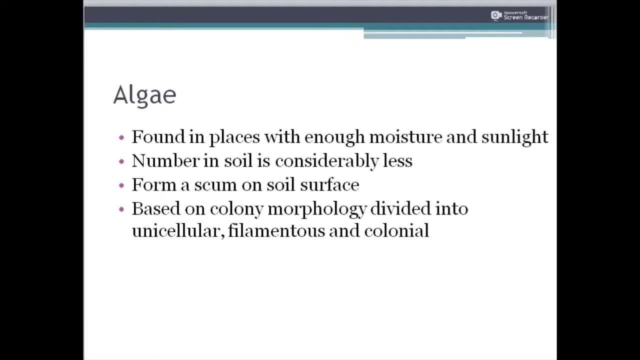 and usually you can see that on the surface of the soil they will form a scum-like structure and usually, based upon the morphology, you can divide them into single cellular forms, filamentous forms or even as colonies. that is, either they will occur as single forms or they will form filaments. you know what's? 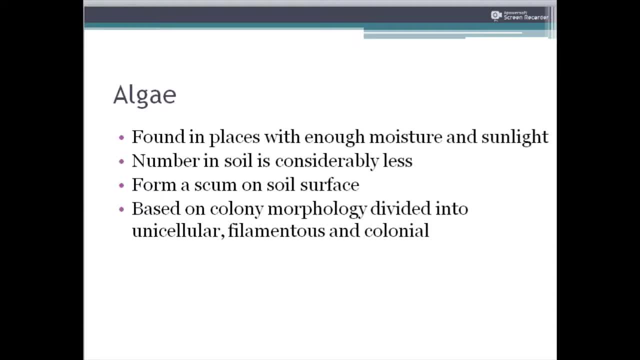 a filament, it's an extended cell or it can be from a colony. a colony is a group of cells which occur together, so algae. they are usually been found to be less in number and they form scums, and they might grow in places where enough moisture and sunlight has only been present. now, if you're going to, 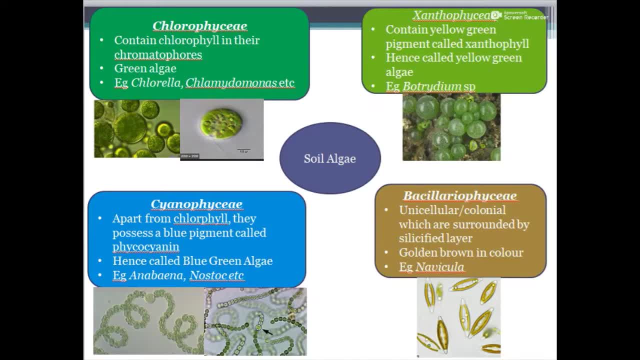 consider soil algae, you can divide them into four different groups. there is a chlorophyse, as the term implies itself. it contains chlorophyll in the chromatophores and it is green in color and hence it is known as a green algae, and different varieties are there. 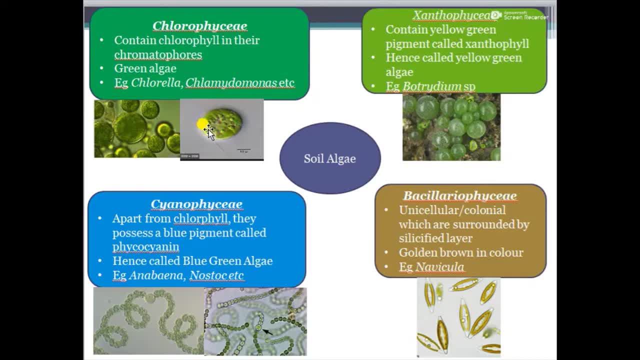 chlorella, as this one, and chlamydomonas. you can see a small flagella also, which has been present over here. so the one group of soil algae is chlorophyze. then the second group is florescent. florescens is also yellowish, green in color, and so you can see this. clowymata is also called xyumorershie and xятьсяphycea. 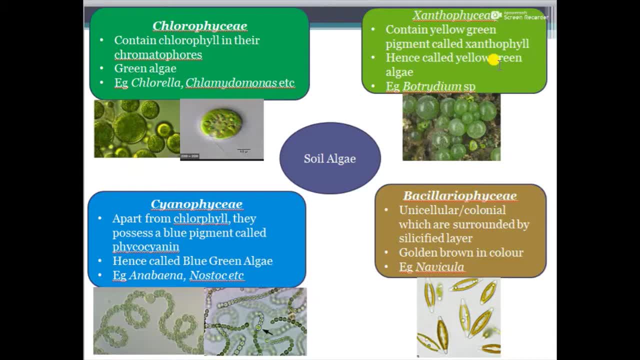 the pigment called xanthophyll has been present over here, and hence we call it as a yellow green algae, and botrydium species is an example of this, and now then we have cyanophyci. you can see that it contains chlorophyll, and also it contains a blue pigment called the phycocyanin. so that is.